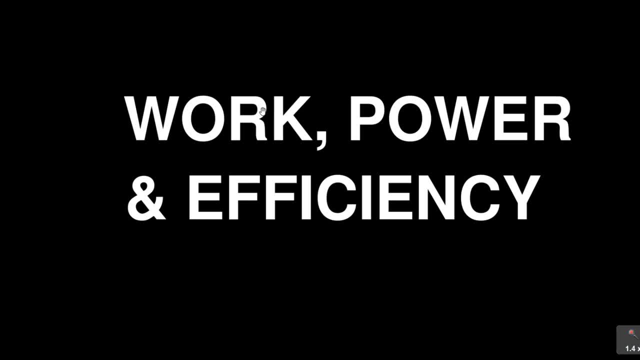 and every work. So for you to do that, I will encourage you to subscribe to this channel so that you can be able to follow up and ensure that the notification bell is turned on, if ever you are subscribing for our YouTube channel. So now let's go through. 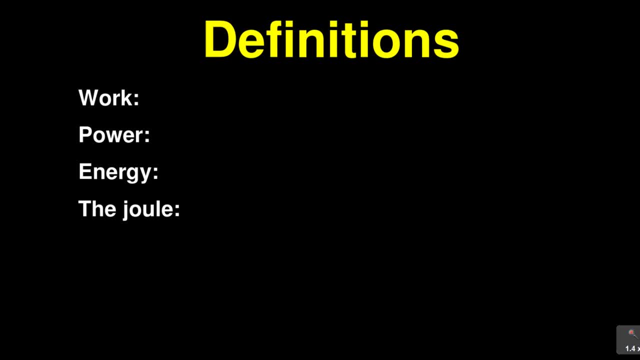 this topic- the work, energy and efficiency. The first important thing are the definitions, and the first one is the definition of what. It is the definition of work. Now, what is work? or what will you define work, as Now? I usually use formulas when I'm defining. Remember, there is a 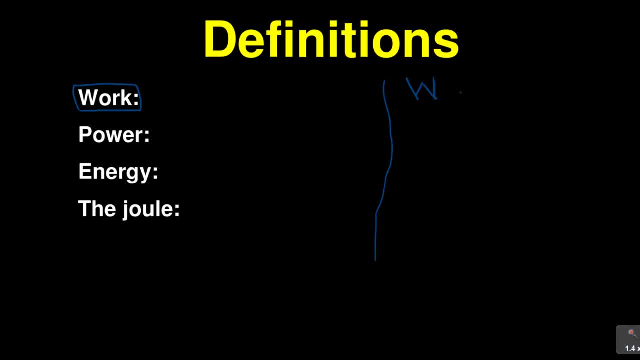 formula. If you go through your formulas, you'll see. this formula says: work is F times S, meaning work is force. F stands for force, S stands for distance. So work is force times distance. Now, how will you define work? Now, work is a force which moves through a distance. So if I talk about 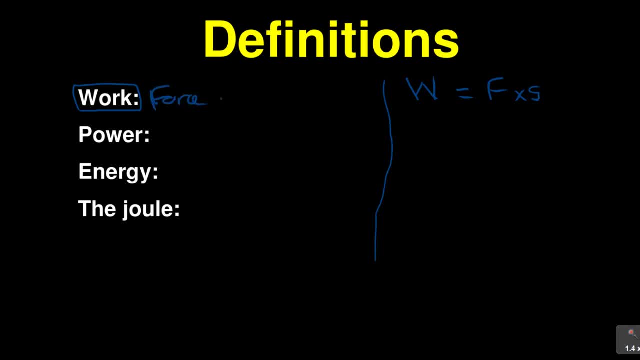 work. we are saying it is a force which moves Through a distance. So that is through a distance. As you can see, it is force times distance. So you're trying to define this definition. So work is a force which moves through a distance. Now, 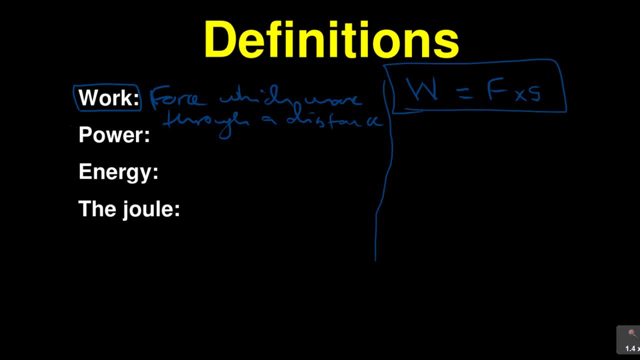 what about power? How will you define this word power? Power is defined as there is a formula for power which says P is equal to W over T. We'll go through this again, but I'm just getting ahead of myself. What is power? Power is the rate. 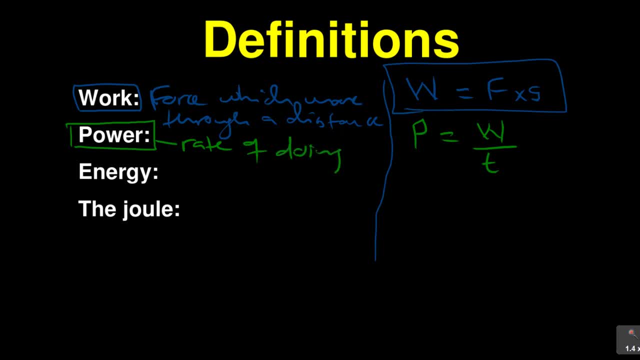 of doing work. So that is that rate. That's why it's divided by time, So it is the rate of doing work. And then the other definition here is energy. How will you define this definition of energy? Energy is the ability to do work. 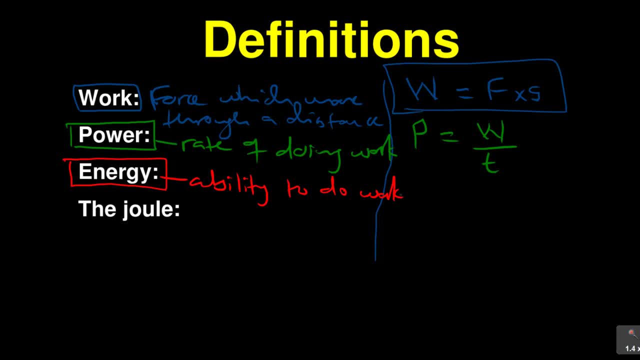 So energy is the ability to do work. So that is energy. Power is the rate of doing work, but the energy is that ability to do work. Now, the unit of work or energy, that unit is the joule. So how will you define a joule? Now, a joule, we can define it as the amount of work done when a 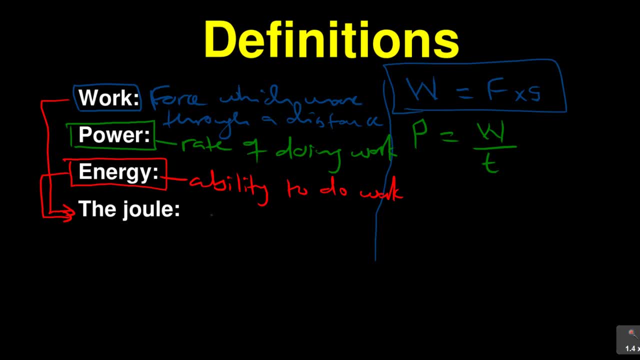 force of one Newton moves through a distance of one meter, So the joule, there we are saying it is the amount of work done. right, That's the work done, remember. And then we're saying when a force of one Newton, as you say, it is force times distance, So moves. 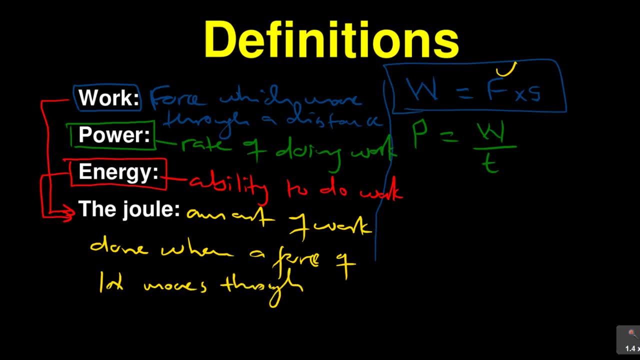 through a distance, through a distance of what? Of one meter. So it's. that's why it's, when you're looking at the joule, it is Newton, Newton meter, It's Newton meter, meaning it's Newton meter. And 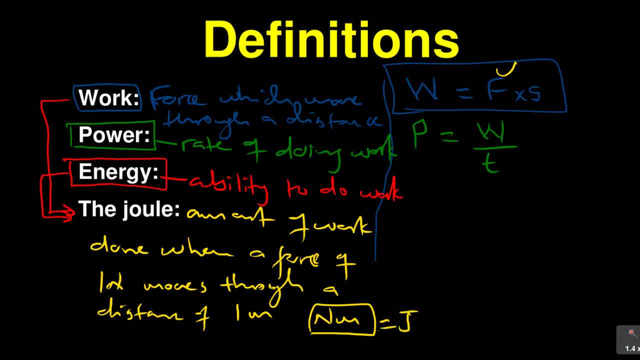 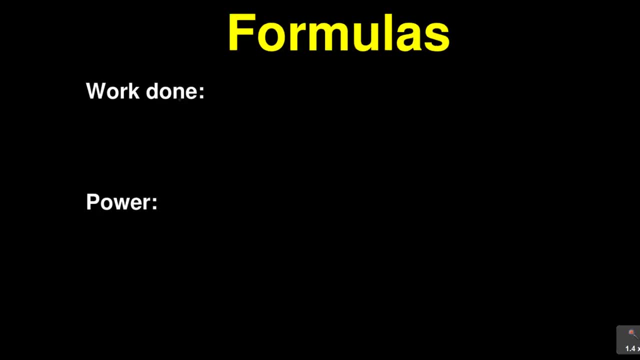 by saying Newton meter, we are saying this is equal to a joule. So these are the definitions that are important for you to know. And then the other definition here is energy. How will you define a joule? Now, moving ahead, let's look at the formulas. As you said, the formula for work done. 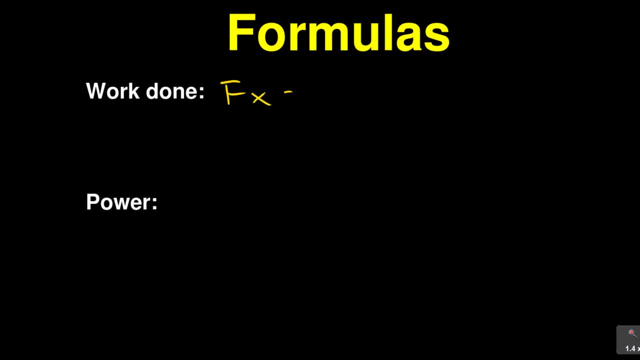 work done is force times distance. Please don't forget that Work done is force times distance. And also, it is important for us to remind ourselves what is force. Now, force, remember, is mass times gravity. So when you're given the mass of an object, you multiply that particular 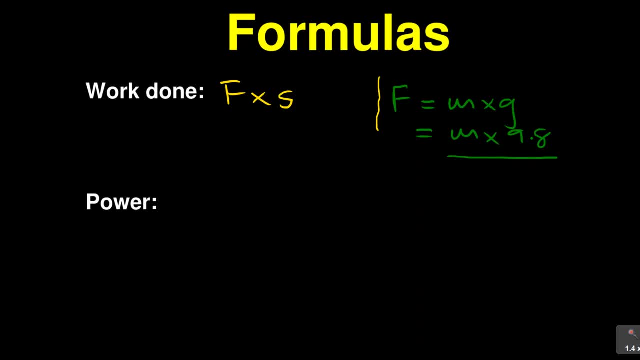 mass and the gravity. there is nine point Now. force times gravity is equal to eight. So we can write now: work done here is equal to force, which is M times G times S. Sometimes you might be needed to use that, What about? 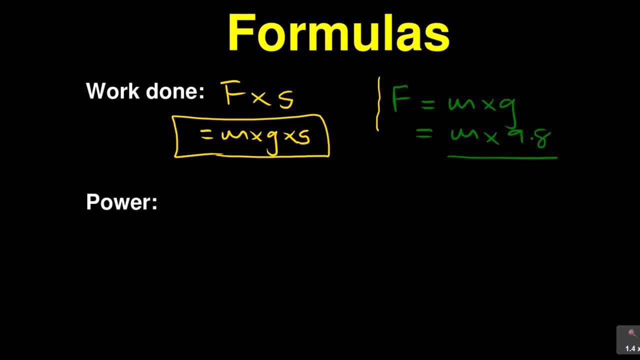 power. We said it is the rate of doing work which is work done. Let me use a different marker here. We said: power is work done over time taken. But now remember work is F times s, So you can actually substitute the way there is work. 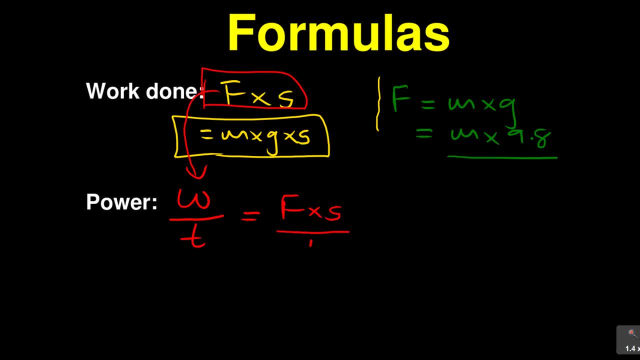 F times S over time taken. that is what you call that. we call that the power. so it is work over time which is force times distance. but now you need to remember what is speed or velocity. now, V is equal to distance, which is S over T. so now you can see that there is S over T there, so we can therefore move on and 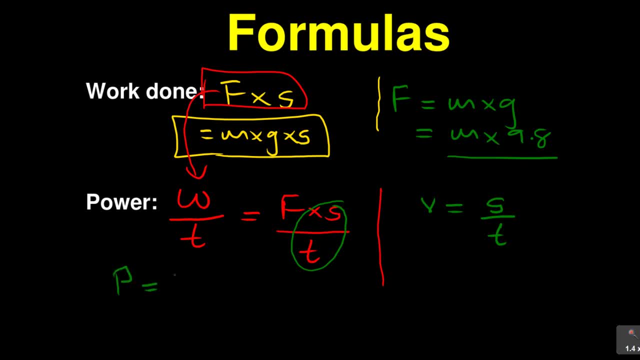 say power, here P is equal to force, which is F times now, since S over T, this gives me a V, so it's F times V. so that is another formula for power. so power here can be work over time, which is force times, distance over time, which is force. 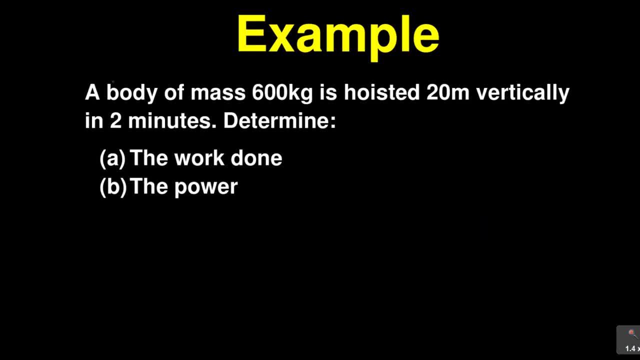 times velocity, depending what you are given. now let us look at a quick example here before the end of the lesson. you can see that there is a power here. P is equal to force, which is F times jcie Amen, and of course, of course, the answer is P. the power of force is V. 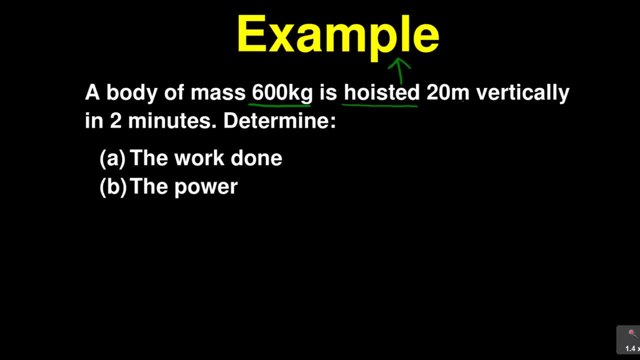 which by definition can be compared to lifting lever that hand from the frame like you hit. okay, so this he's saying: a body of mass 600 kg is hoist. it to hoist is to move vertically up 20 meters vertically into we need determine the work done. so this is just a simple example here to say how. 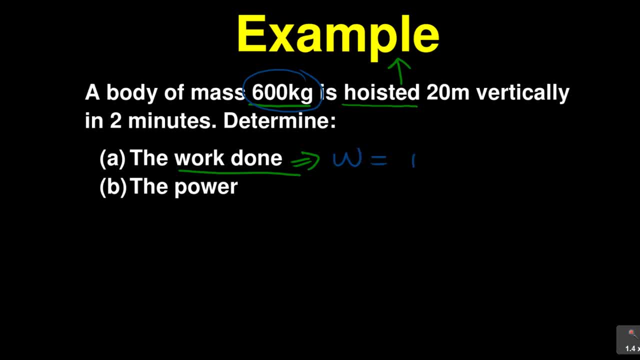 equation says: calculate the work done. remember work is force times distance. so we have s here. this becomes our s for the distance. but what about our force? our f is linked to that 600. so remember the formula i said to say you need to convert the mass to newtons. so we are saying what? 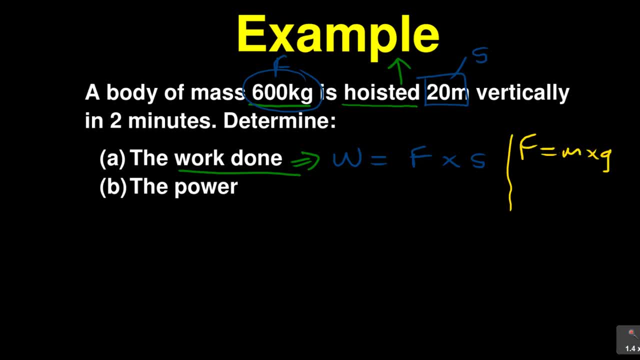 f is m times g. so what do we have for the mess? which is 600 times 9.8. so you can take that and say work now is equal to- you can actually find the answer here first- which is a, what is 600 times 9.8, and um, the calculator can give you, uh, an answer for that. so it will be 600 times 9.8. 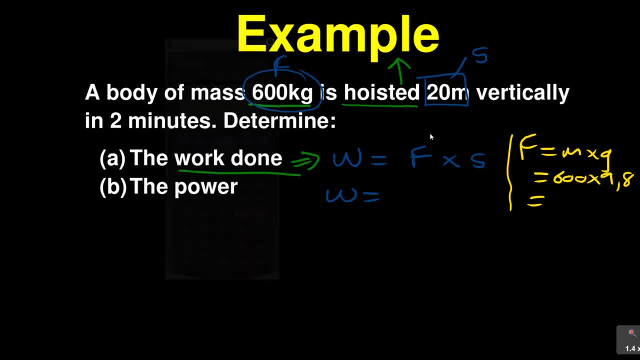 if you're going to simplify things is 5 8, 8, 0, that's what you'll have here- 5 8, 8, 0, that is now in newtons. then you can take that and say 5 8, 8, 0, now times distance, which is 20, and then you're going then. 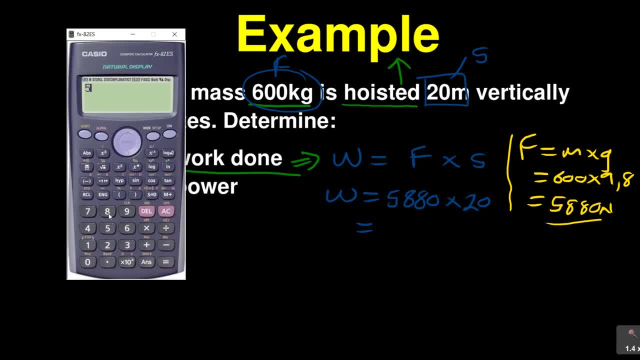 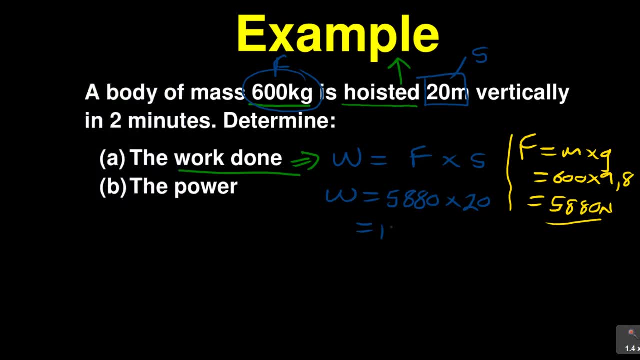 to get the answer in this case, to say 5, 8, 8, 0 times 20, then this becomes 117, 600. now what are we looking at? work done is measured in joules. you can divide by a thousand. it would be one one seven comma six. then you can convert it now into kilojoules. but that answer is the standard. 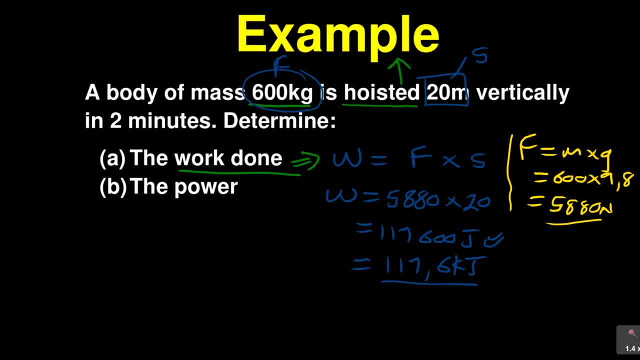 form. now that was a. what about b? in b, what are we calculating the power? how will you calculate the power now? remember, we said power is what work done over time taken. now we're going to take the h function of the time that we saved and remove our character from the power. let's just say r over. 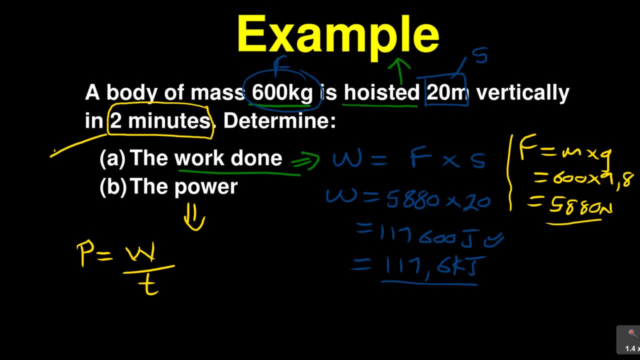 here we're taking a number and understanding what the total time has to do with the number of days my plot or to do what i'm doing, it initiating right now is zero and i'm going to give me a was nice weakness here. and if you would just to help me, if you go to my reader and look at 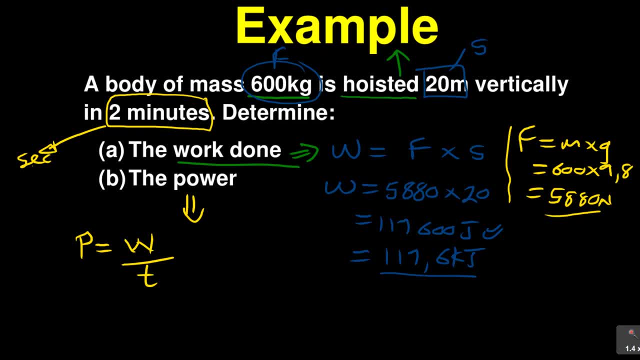 some of the announcements here. i have prepared the plot, of course, which is Lockheed Martin and really daring move on to that. i wanted to explainicki loop and how to convert that rokwore unit of timeOk now let me say this: okay, so here's what we're doing if we converted something. 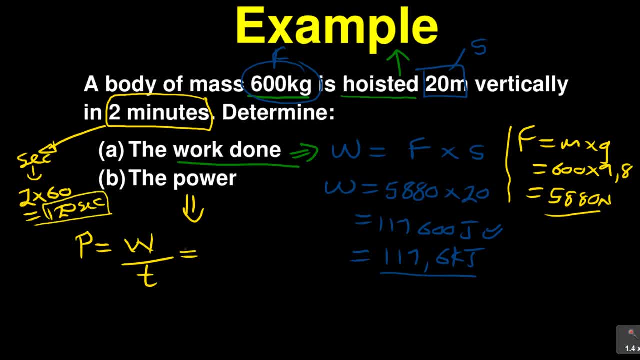 that part. so when you say power is equal to wet done, we just got the wet done here, which is 117 600 over time. now, don't forget the SI unit of time is in seconds- then it's 120. then when you do that, again, as I said, you need the help. 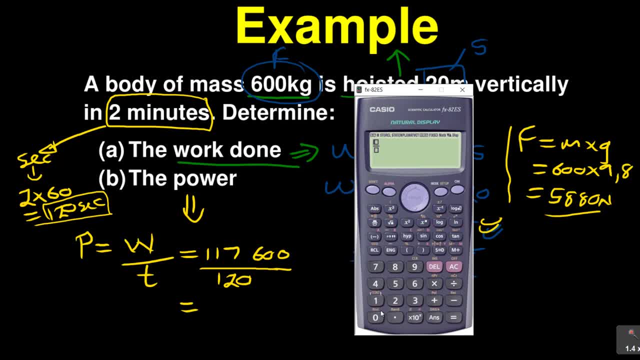 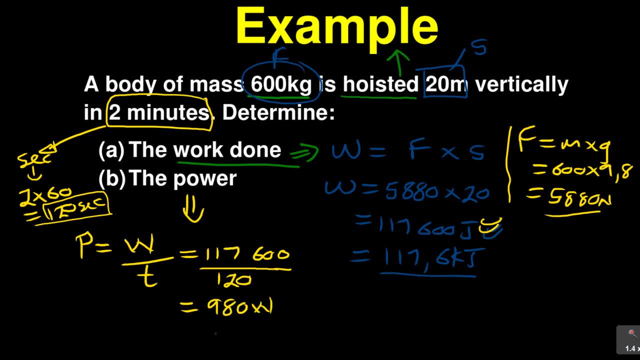 of the calculator. if ever you're looking for to say one one seven, six hundred over 120, then it will give us 980. so it's 980. now, power is measured in watts. that was one way of doing it, but I say as I said, there are different formulas. 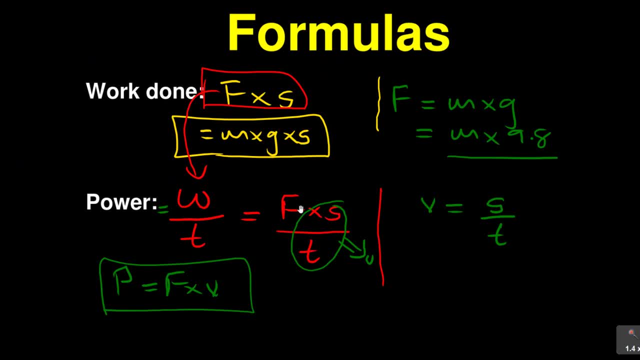 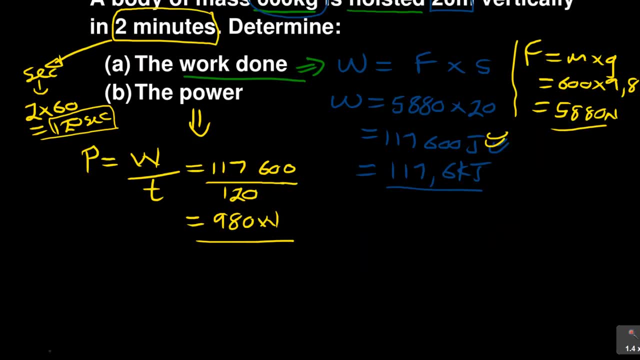 that you can use and we said. another formula for power is: is this formula here the? this formula here is F times s over T, so you could have actually used it here to say: power is equal to F times s over T, which is equal to the force we did find. 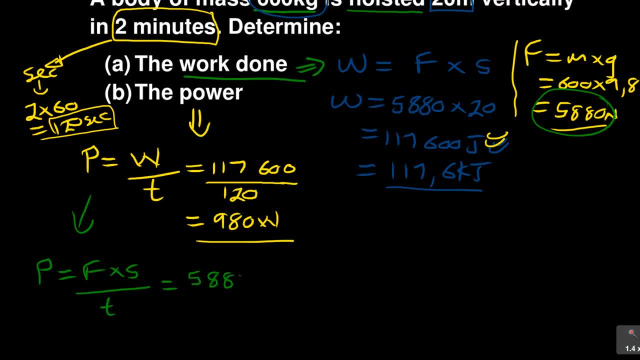 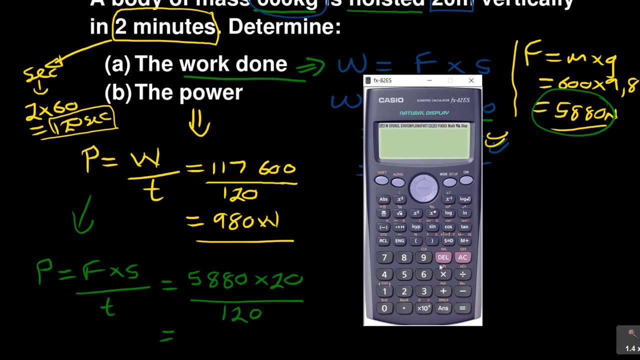 F here, which is 5880 times the distance, which was 20. see that over time, we say to remember, is 120 seconds. so this can actually give you, if you are working directly from before you calculate the wet add work done, which is eight, eight zero times 20 over 120, then you can see that it's 980 stretch. so 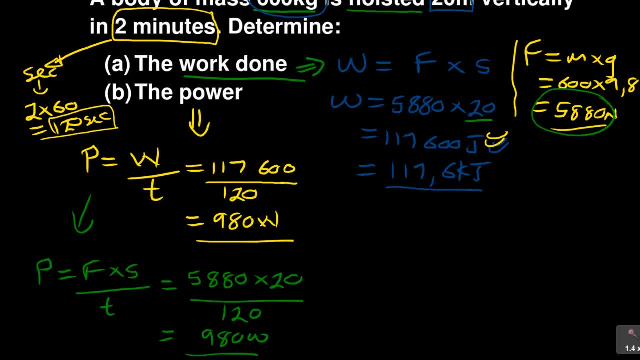 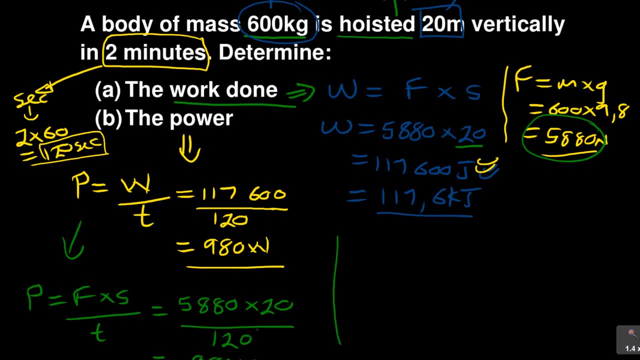 it's got nine hundred and eighty watts. so depending how you want to do it, this can be different ways of doing it. and let's see here they are saying all. you can actually look at it from this angle to say velocity, remember. you can actually look at it from this angle to say velocity, remember. 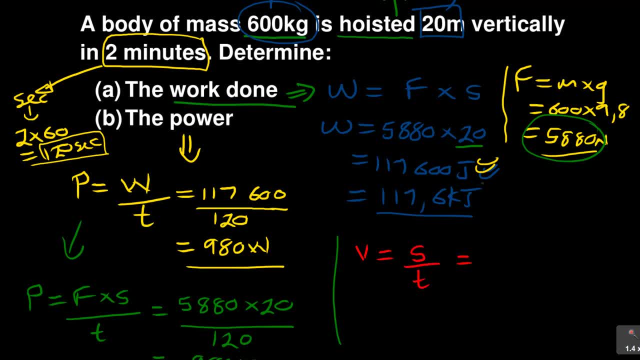 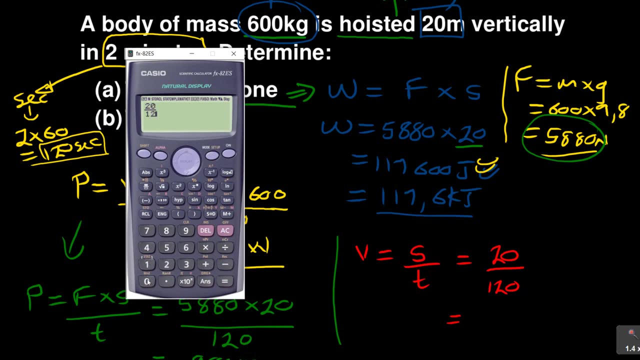 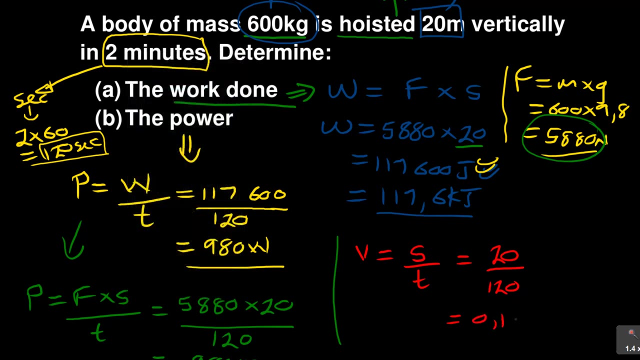 is distance over time, and they gave us distance which is 20 meters over time. in seconds is 120. so we can actually calculate the velocity there to say what is the velocity which is 20 over 120, and then i'm getting what? uh, 0.1667. so it's equal to 0.1667. this is meters per second. then 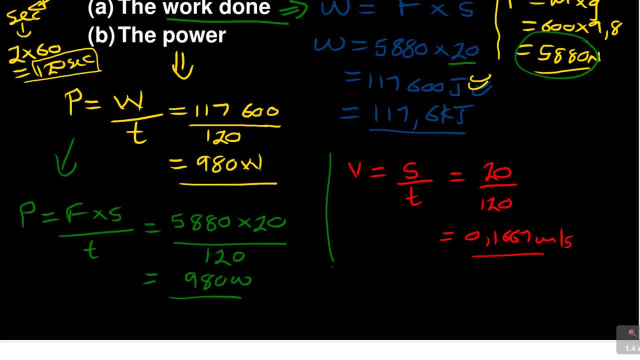 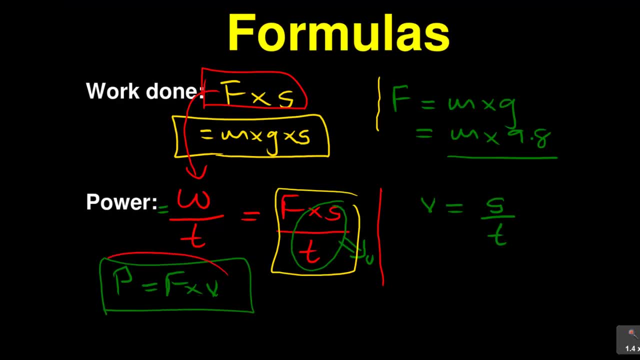 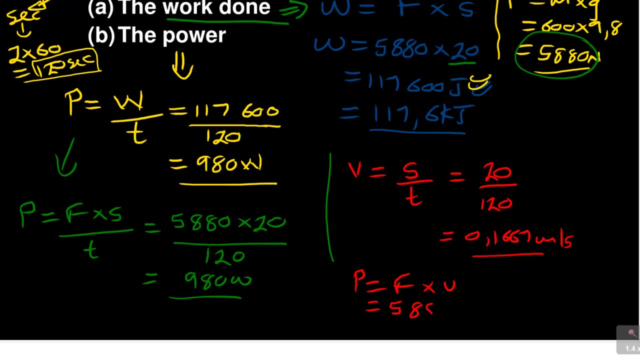 i'm going to take that to say power is equal to f times v, remember we used, uh, that power there, that formula, the f times v, which is equal to the force. as you say, it is five, eight, eight, zero times zero, comma: one, six, six, seven. now to get the actual answer, it was one over six, remember? this was like? 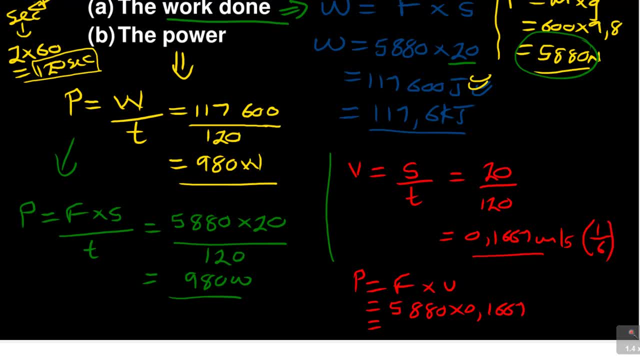 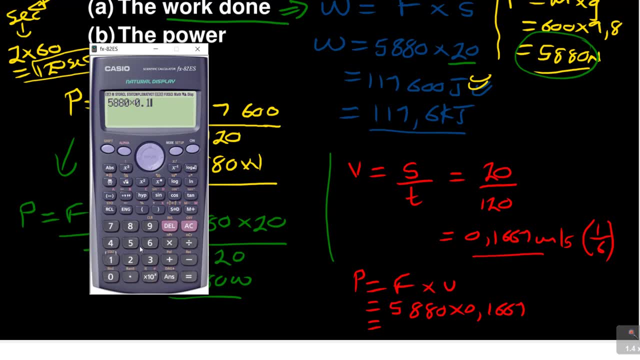 one over six, so that you can get the actual answer. so it is f, which is five, eight, eight, zero times zero. comma one, six, six, seven, and then, if you do sdc, 980, comma one, nine, six, but if i use this one to say times, uh.